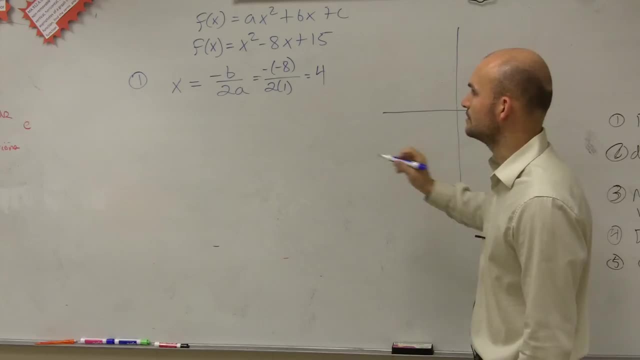 Questions: Okay, Where did I get 2a? That is the formula for axis of symmetry. That was in your notes. we took last class period, So I'm going to draw this nice little dotted line because I remember that the axis of symmetry 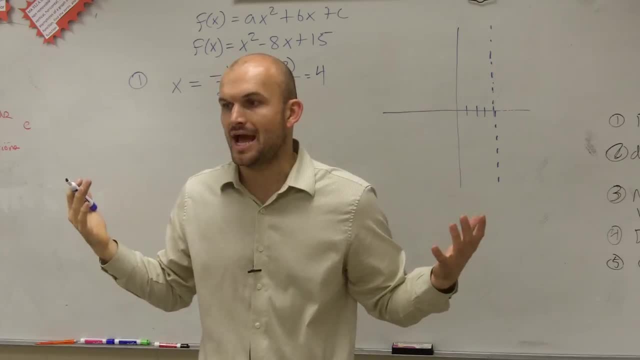 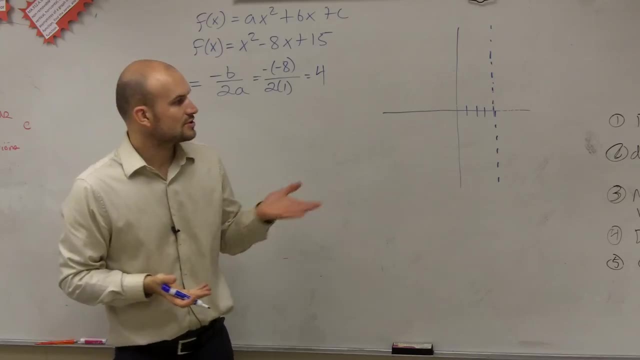 is going to be the line That's going to split my graph into two congruent halves. Right, Yeah, Alright. So now I just need to determine some points. So the next thing is make a table of values and determine. I choose for you guys. 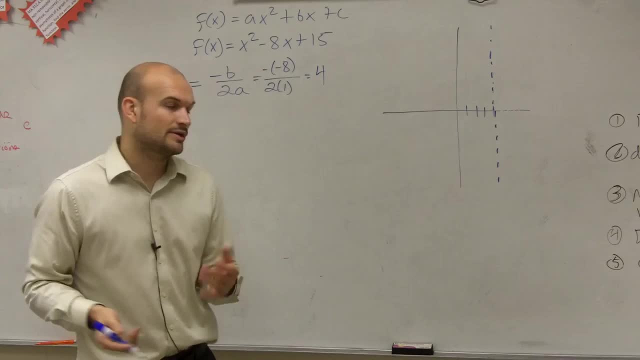 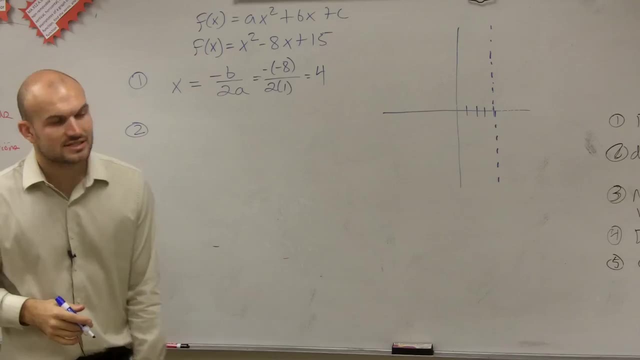 to determine at least two points to the left and two points to the right. So we created a table of values. So, uhm, oh, I'm sorry, actually, before I do that, Sorry, I'm skipping ahead Step. step number two is determine up our graph: opens up or opens down? 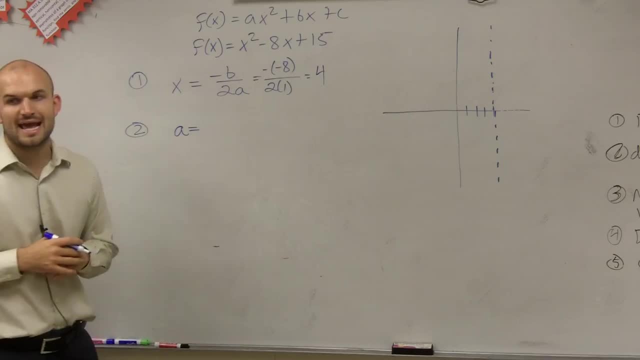 So what we need to do to determine that. determine, that is, we need to determine what a is. a is equal to 1.. So, therefore, a is greater than 0, right, As 1 is greater than 0.. So, by looking at your previous notes, when, 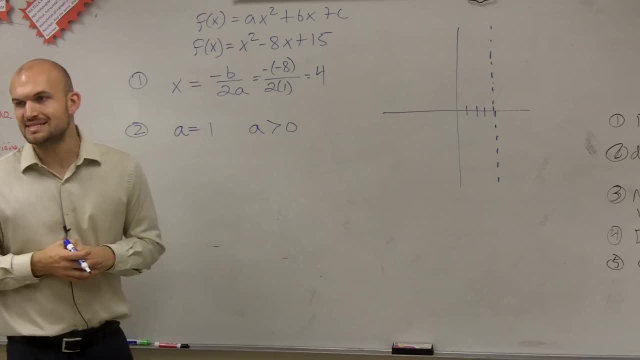 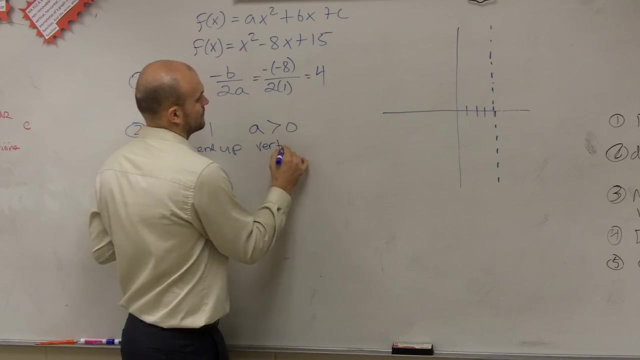 a is greater than 0, your graph is going to open up or open down. Open up, So your graph opens up. Therefore, your vertex is going to be a maximum or a minimum. So you guys now know that your graph opens up. So you could kind of put arrows right there. It's. 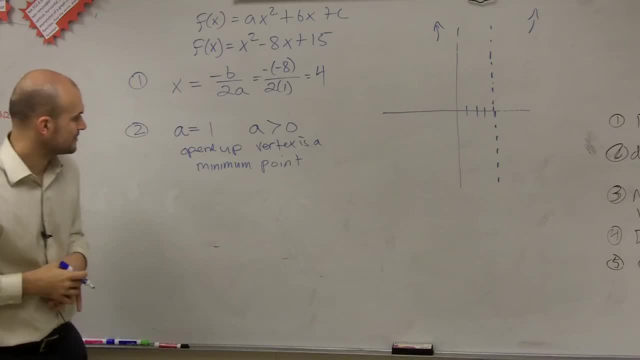 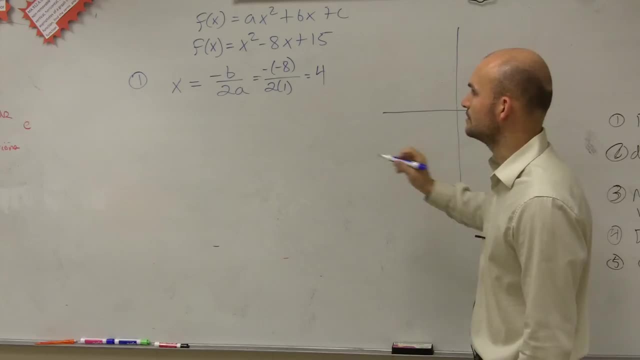 Questions: Okay, Where did I get 2a? That is the formula for axis of symmetry. That was in your notes. we took last class period, So I'm going to draw this nice little dotted line because I remember that the axis of symmetry 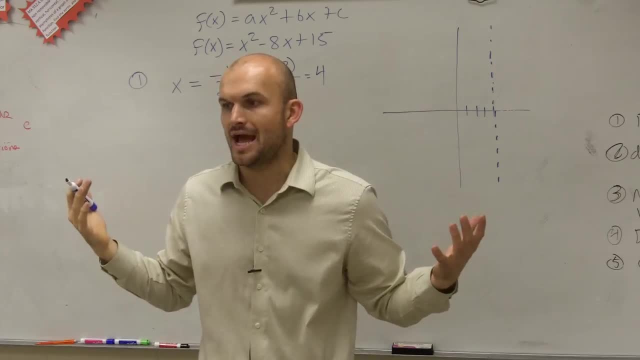 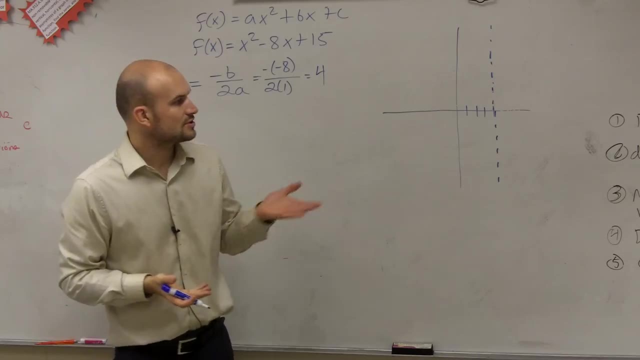 is going to be the line. So I'm going to draw this line that's going to split my graph into two congruent halves. Right, Yeah, All right. So now I just need to determine some points. So the next thing is make a table of values and determine. I choose for you guys to determine. 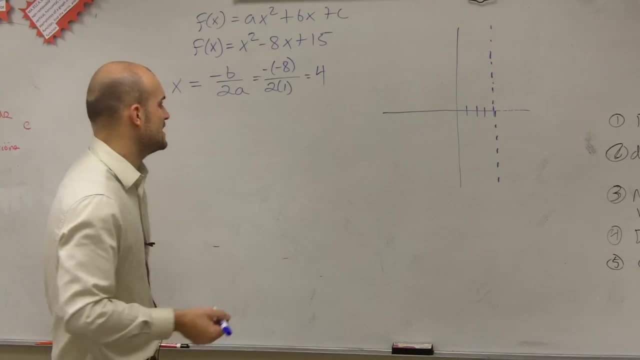 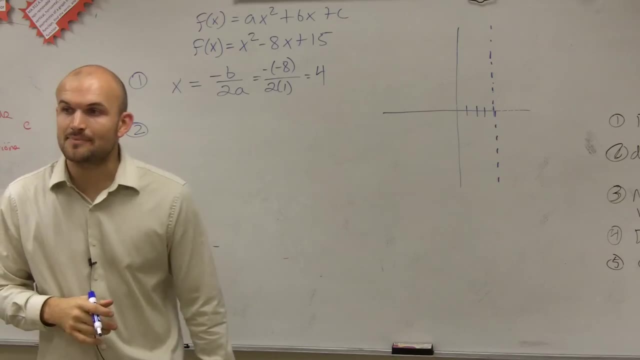 at least two points to the left and two points to the right. So we created a table of values. So, um, oh, I'm sorry actually, before I do that, sorry, I'm skipping ahead. Step number two is determine if our graph opens up or opens down. 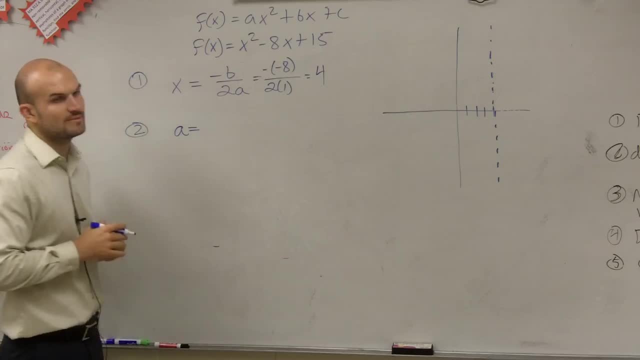 So what we need to do to determine that is So. we need to determine that is So. we need to determine that is, we need to determine what a is. a is equal to one. So therefore, a is greater than zero. So therefore, a is greater than zero. 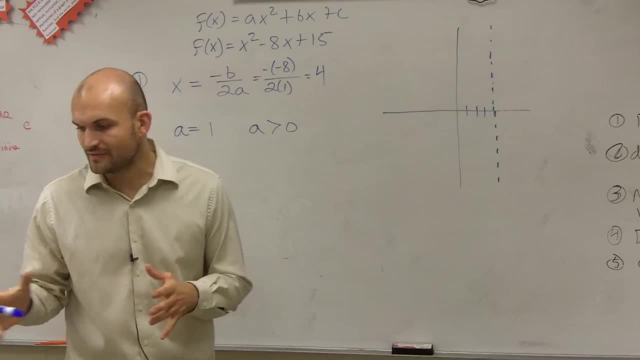 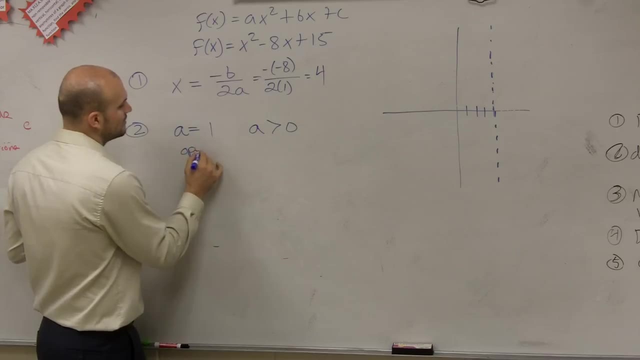 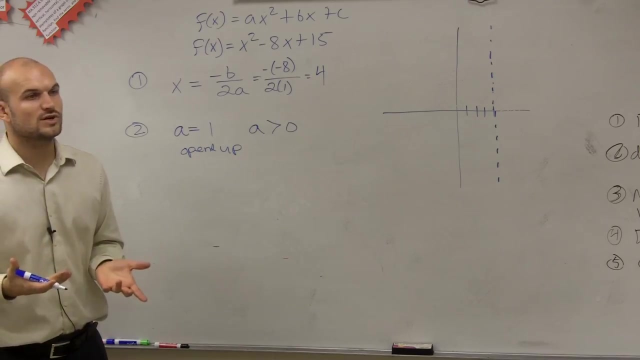 Right, As one is greater than zero. So, by looking at your previous notes, when a is greater than zero, your graph is going to open up or open down. Open up, Open up, So your graph opens up. Therefore, your vertex is going to be a maximum or a minimum. 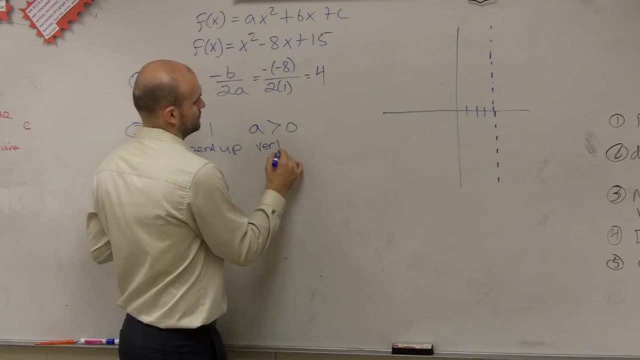 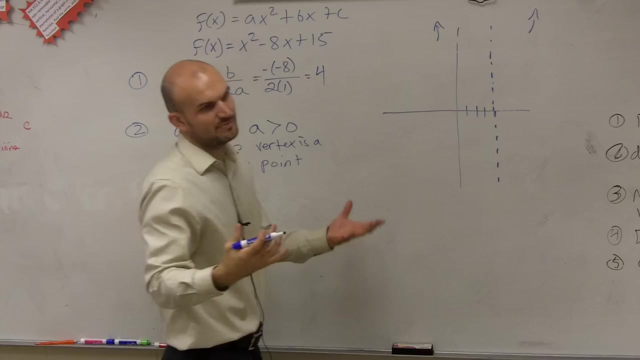 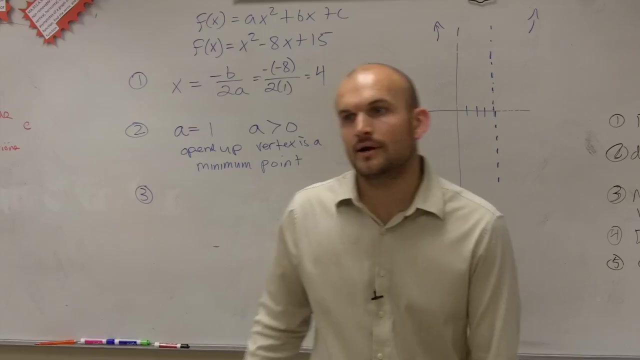 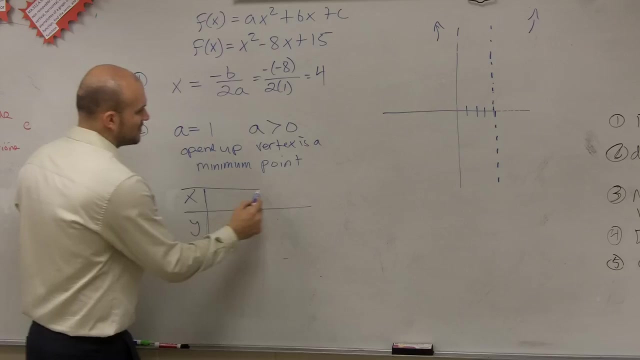 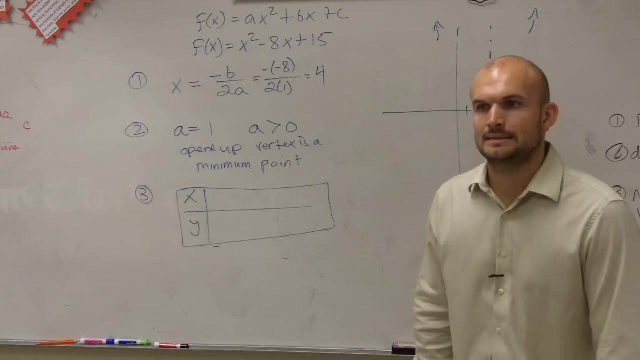 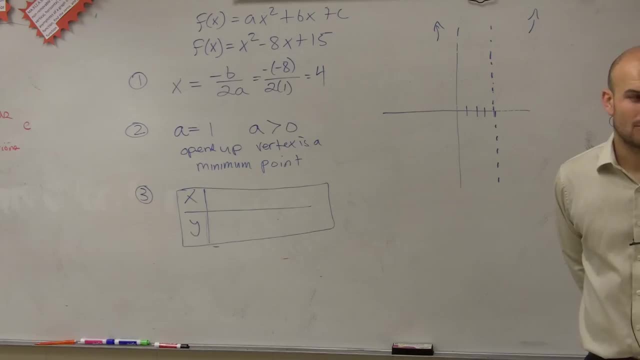 Anybody remember from last class period? What does the x value of your vertex have to do with the axis of symmetry? Yes, Oh, I'll start. Alright, so it's the x, then it's the x line of symmetry, Right? Remember, ladies and gentlemen, your vertex has to, or your axis of symmetry goes. 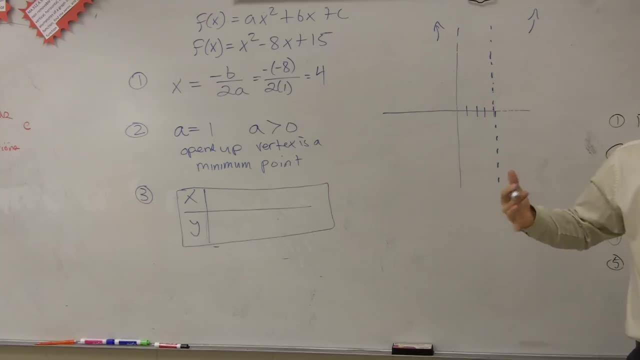 through your vertex, Right Your vertex. your axis of symmetry goes through your vertex. That means my vertex has to be on this line. So the x value of my vertex is what? Four? So I'll just pick 1.4.. Alright, Now what I'm going to do is you guys can do the table. 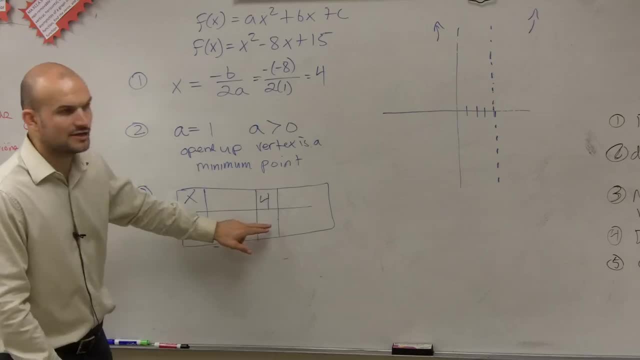 of values. and let's so. if I know my x value is 4,, how do I determine my y value? And we're actually talking about a function, so instead of y values, I'm going to say f of x. So if I know my, if I know x equal to 4, how do I determine what my f of x value is going? 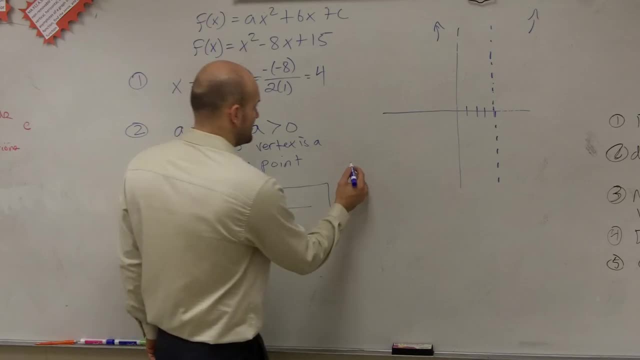 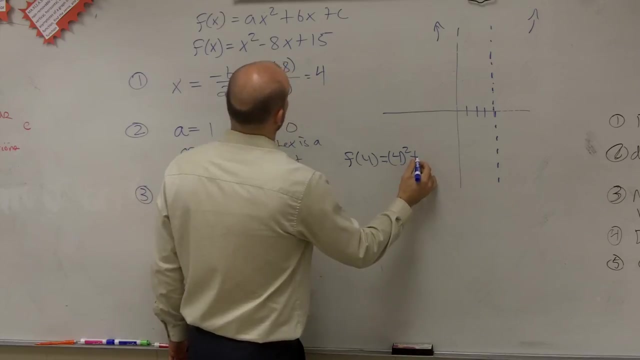 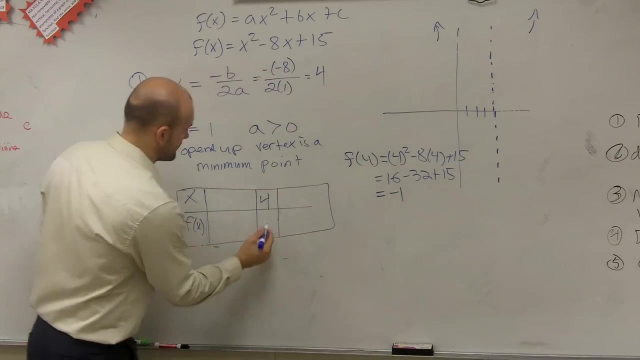 to be. You plug it in, right, So you could say: f of 4 equals 4 squared plus- I'm sorry- minus 8 times 4 plus 15, which equals 16 minus 32 plus 15.. Which equals negative 1.. Right, So your vertex is at 1,, 2,, 3, 4, negative 1.. 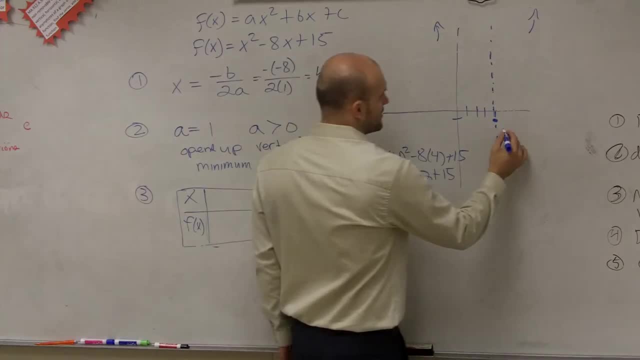 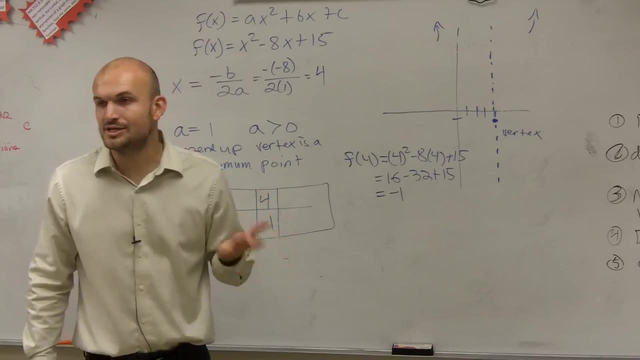 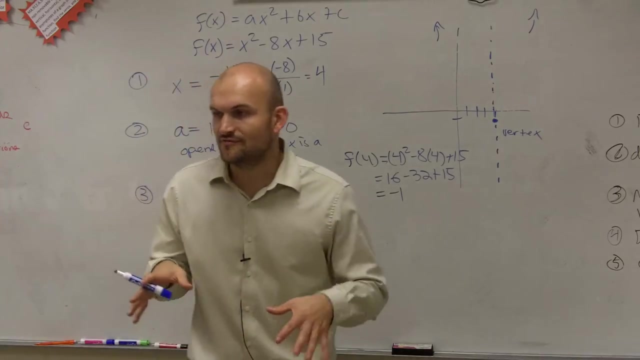 Does everybody follow me with that? So I'm just going to label that vertex. Okay. Now here's the next part that you guys can make easier or harder on yourselves, Alright, Really, depending on what you want to do, I chose, I set in my directions to find two points to the left and two points to the right. 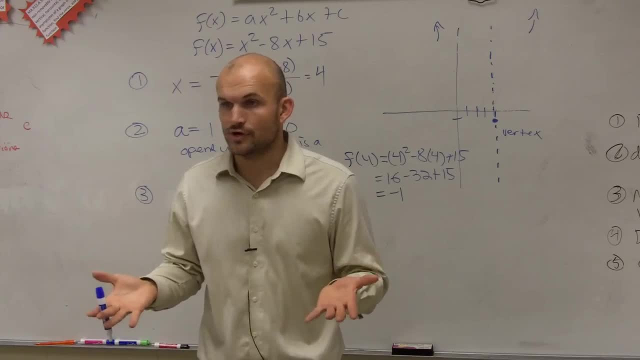 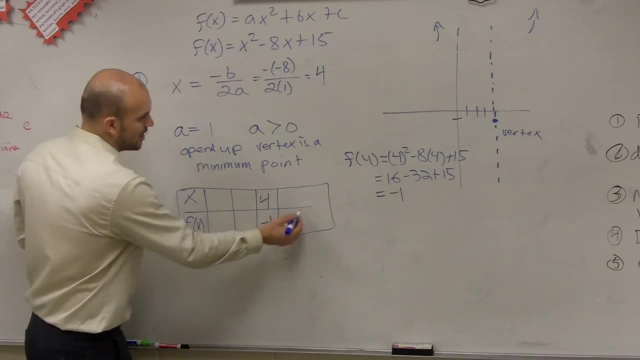 I don't really care which one you do first, but try to find at least two points to the left and two points to the right. Then I'll show you guys a shortcut. So what would be two points that are to the left of my axis? symmetry. 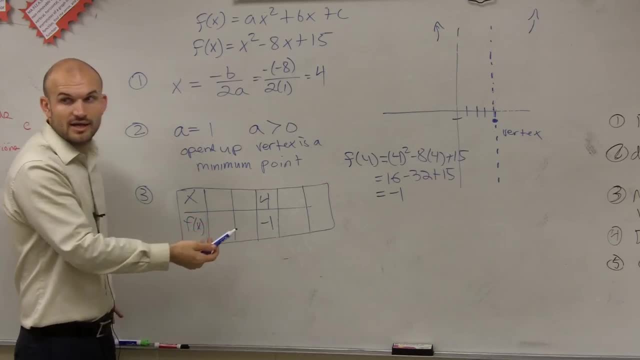 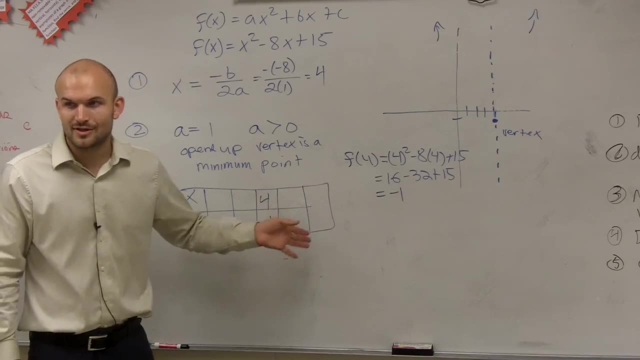 You could do 3,, 2, right. You could do like negative 10, negative 20,, Madison, If you do two negative 20.. Well, ladies and gentlemen, my advice is try to do points that are very close to your vertex, because the quadratic gets pretty large, pretty quickly. 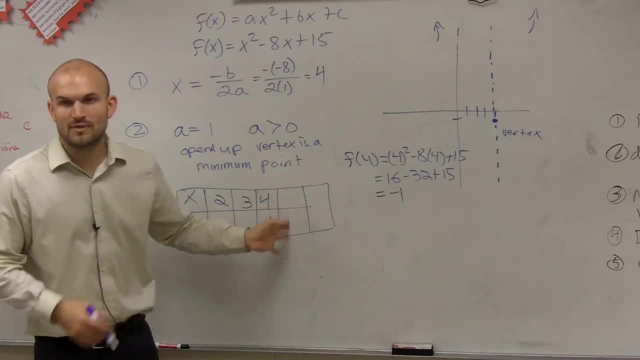 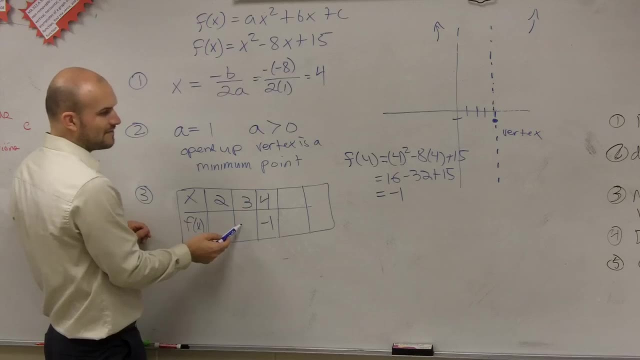 So I'm going to pick the points 3 and 2.. Now you could say, Oh well, that could be 5 and that could be 6. but before you do all of the work, let me show you a little tip that you can do. So if I want to find now the f of x value, I do the same thing.